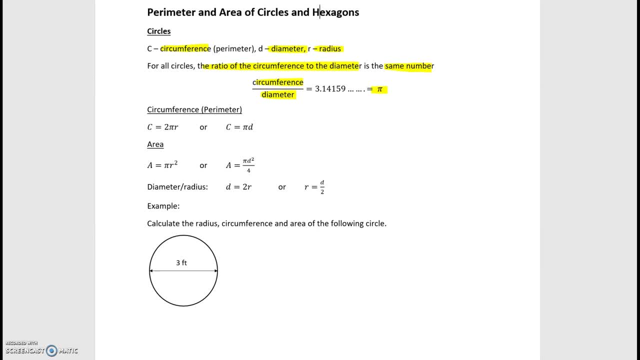 probably come across pi before and most commonly know it as 3.14.. Some people have more than two decimal places memorized, but 3.14 is a very common, known measured value for pi. Okay, so let's take a look at how to calculate circumference. So circumference- and we know that the 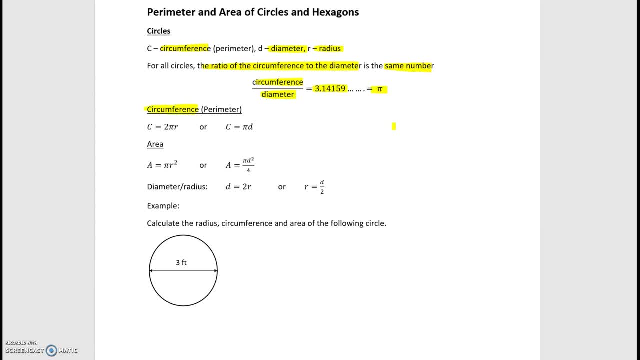 distance around the circle, or in other words perimeter, but most commonly used as circumference, is calculated as 2 pi r, 2 times pi times radius, or, because we know radius is half of the diameter, pi d. We'll also be looking at how to calculate area of a circle, So that is a common formula. 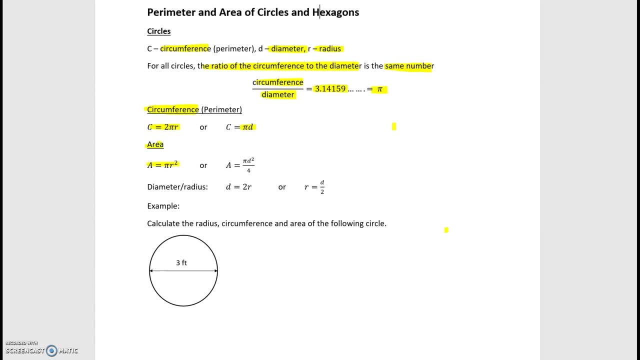 which is a equals pi r squared. There's a little more technical one as well, which is pi d squared over 4, but we're going to use probably pi r squared. And lastly, remember the formula for diameter: Diameter is twice the radius. or, if you were to rearrange that, which we'll be doing, more algebra in the course in a bit. 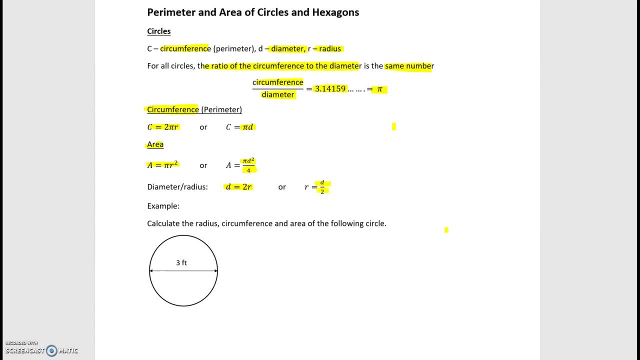 radius is equal to that diameter divided by 2.. So now we're going to take a look at calculating the radius, the circumference and area of this following circle. So we're going to take a look at the following circle. Okay, radius is equal to diameter divided by 2.. The diameter in this case. 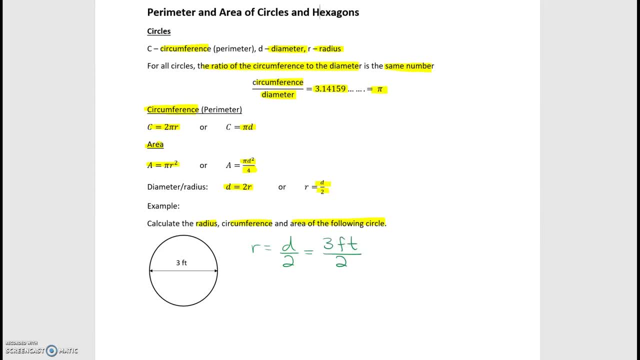 is 3 feet divided by 2, right, This is your diameter, and so that's 1.5 feet, Easy enough. Next, circumference is equal to: we can pick either formula 2, pi r or pi d, since we have both pieces of information, So I'll go with pi d. So that's pi times 3 feet, and 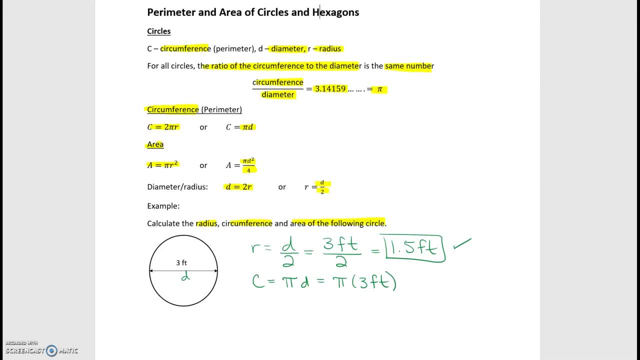 I'm going to use my pi button on my calculator. It's okay if you use 3.14 as well. just pay attention to the instructions on your assessments to see what you should be using. So this one in my calculator works out to 9.42 rounded to two decimal places. I'm just choosing to do that. 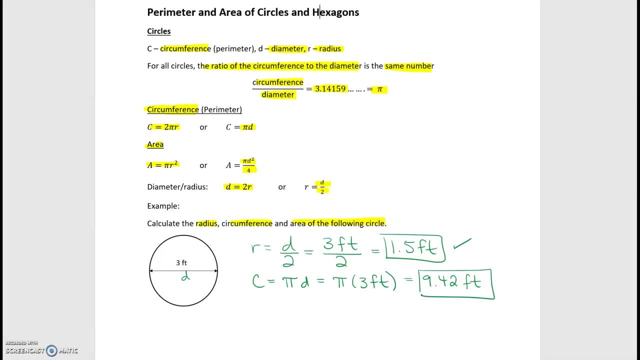 and feet Is my answer. It's just a distance around, So that'll just be a straightforward feet answer. And area is equal to. I'm going to go with pi r squared. Could have done pi d squared over 4, but this one is more commonly used, or commonly known, So pi times 1.5 feet. 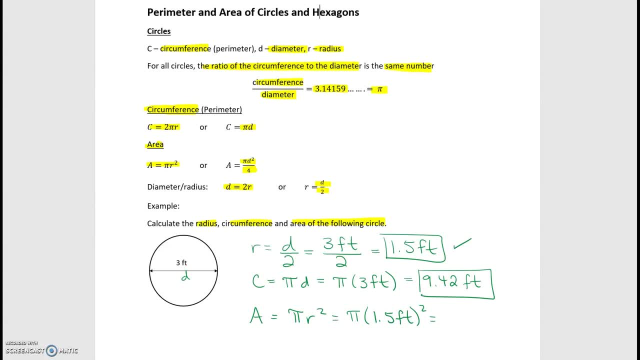 squared. Be careful of your units. It's area, So that squared applies to the 1.5 and the feet. So putting that into my calculator I'm doing: pi times 1.5 squared and rounded to two decimal places gives me an answer of 0.07 feet squared. 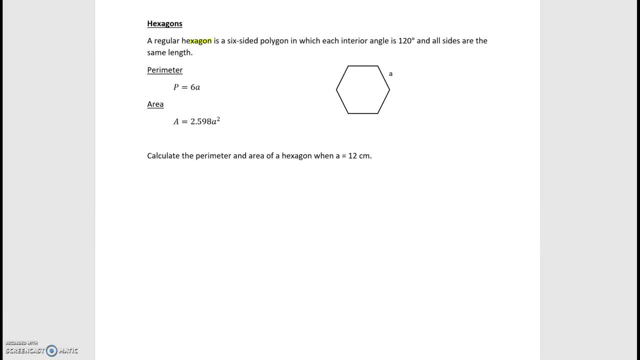 Next we'll look at hexagons. Well, a hexagon is a six-sided polygon, a six-sided closed shape in which each interior angle is 120 degrees And all sides are the same length. So here's a perimeter formula for a hexagon: six sides. 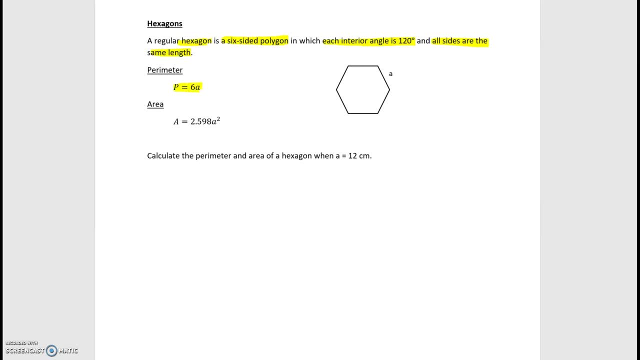 perimeter equals six sides of the A value. Okay, The area formula is something very specific: 2.598 times a squared. So let's calculate the perimeter and area of a hexagon. when A is 12 centimeters, perimeter equals six A. In this case, A is 12 centimeters and A is 12 centimeters. 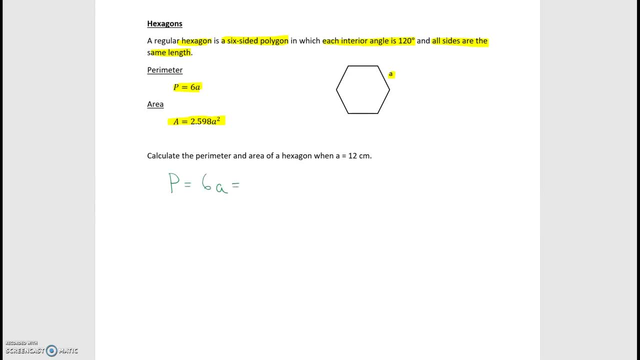 So I'm going to add that to the square of the hexagon, which is 4.9,. so 2 and 5,, 7 and 5.. So is 12 centimeters. This works out to a nice whole number of 72 centimeters And using the area, 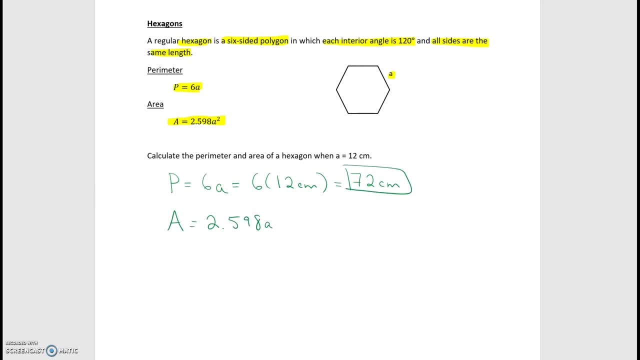 formula 2.598a squared. So remember, just like the example above, everything inside the bracket is going to get squared, The 12 is going to get squared and so is the centimeter, which is why you have squared units, always for area And this one. I'll just display all the answers. Oh, 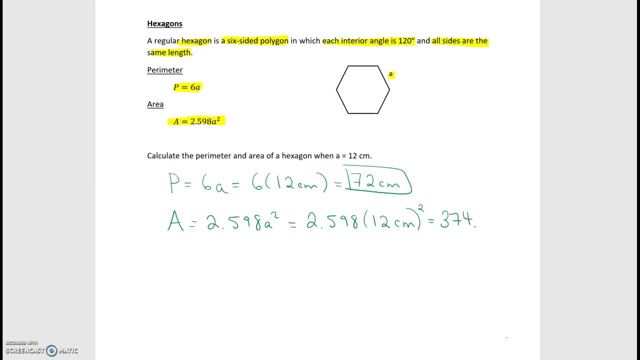 there was a 4. 374.112 centimeters squared.